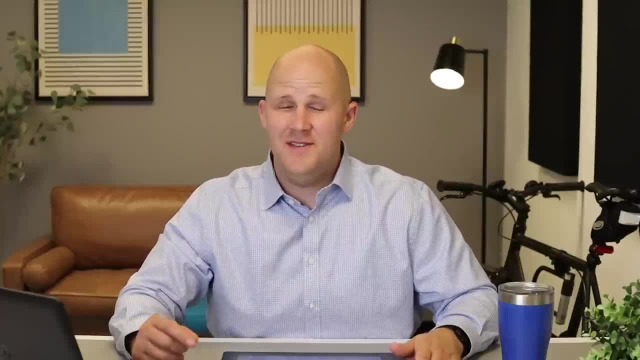 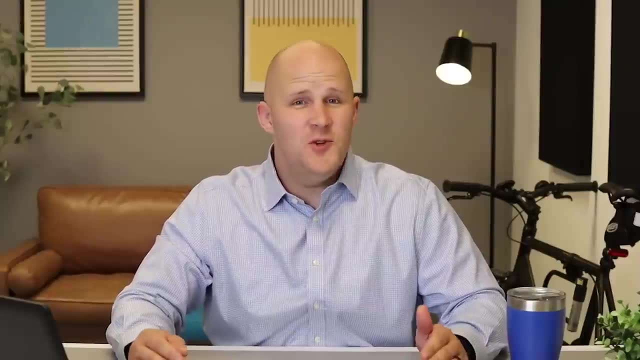 And follow right along with me. Plus, as a bonus, I'll show you where you can download this free cheat sheet that's going to help you choose the right chart every single time. I promise you that by the end of this crash course, if you truly pay attention and try to apply the learnings, 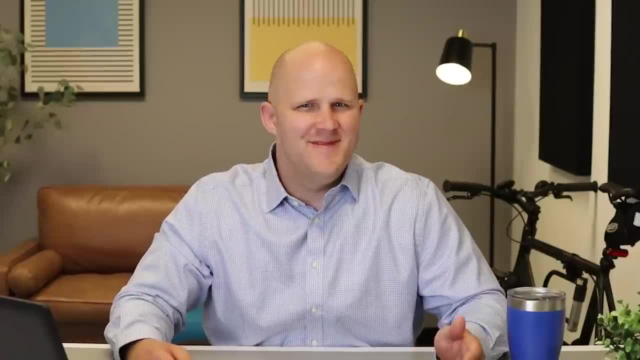 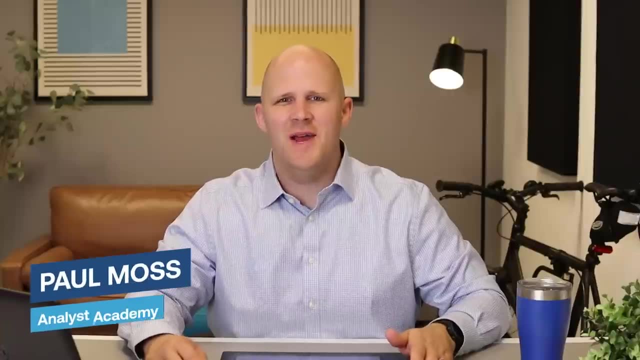 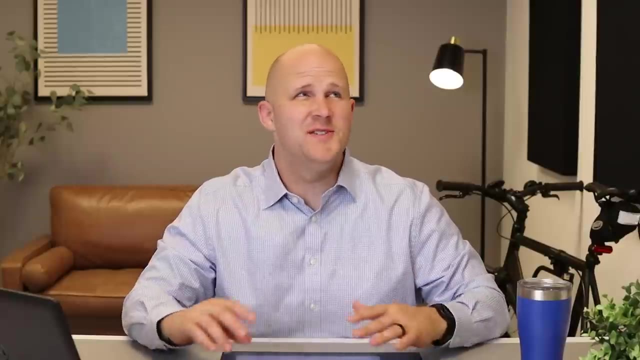 you'll be amazed at how much more effectively you can communicate data. Let's get into it. Hey everyone. Paul here from Analyst Academy, where we teach PowerPoint, presentation design and data visualization training, to consulting firms and finance teams and all sorts of other teams all over the world- If that sounds like something. 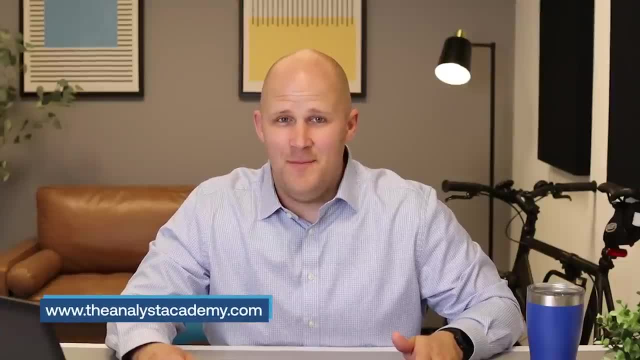 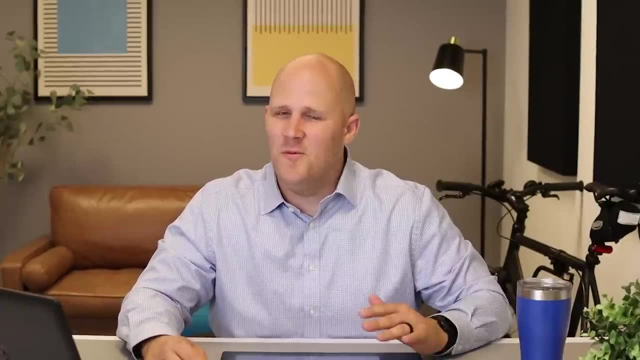 you're interested in, make sure you check out our courses over at theanalystacademycom. And if you're watching this video, you might especially be interested in our data visualization for consultants course. It's kind of like this video but way more detailed with hands-on. 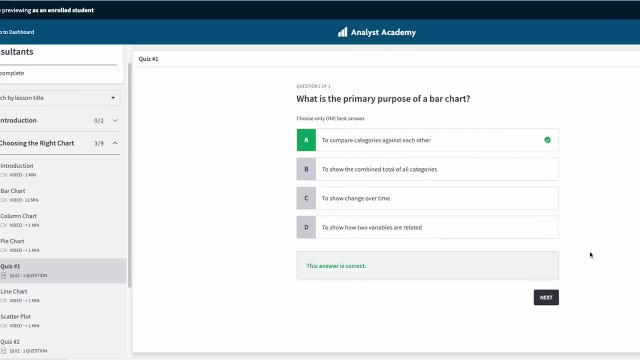 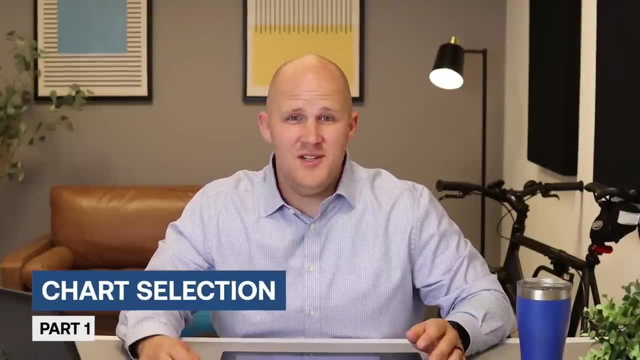 exercises, case studies, quizzes and a whole lot more. So make sure you check that out Again. that's theanalystacademycom. The first and most important part of effective data visualization is choosing the right chart type. To illustrate this, let's take a look at the example from the beginning of this video. 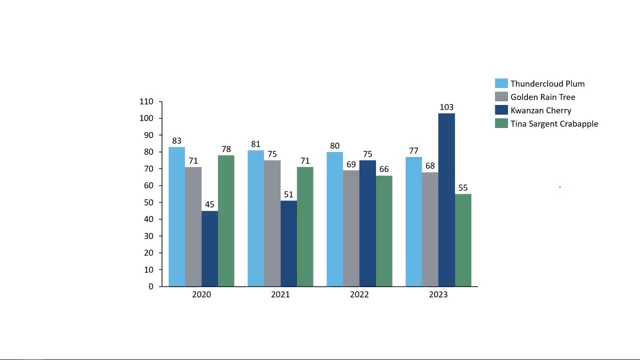 Once again, this is showing tree sales for a local nursery. So you've got your four different tree types here, and it's broken out into different clusters based on year. This is what's called a clustered column chart. The takeaway for a chart like this might be something. 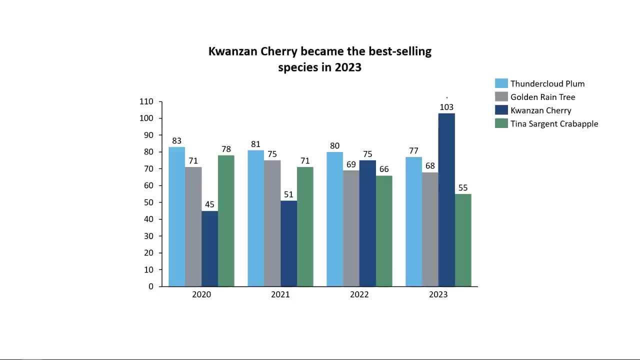 like Kwanzaan cherry, became the best-selling species in 2023,, which you can clearly see right here. You're comparing each of these different species against each other, And in 2023, is when it first became the number one selling tree. But then what if you put the data in? 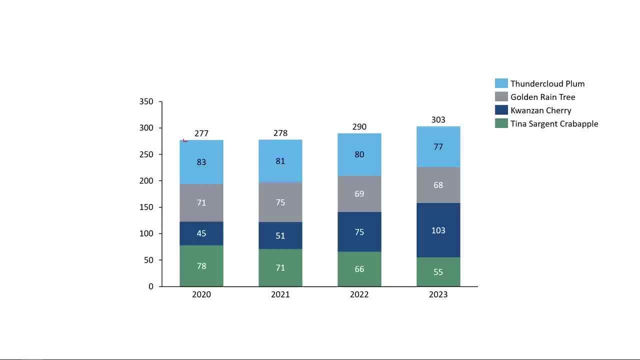 a stacked column chart like this. Now the emphasis seems to be on the total of each of these columns. You're combining all the species together, so the focus gets put right here on the overall total. So a message for a chart like this might be something like: 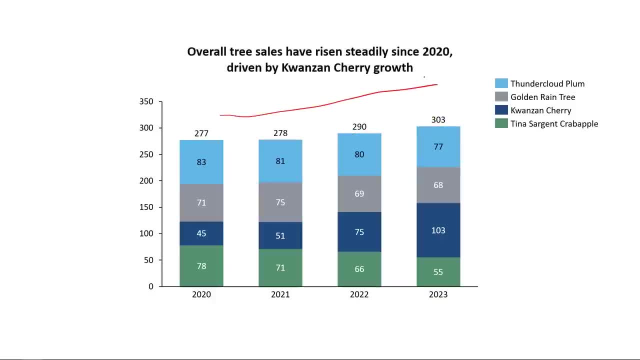 overall tree sales have risen steadily since 2020, driven by Kwanzaan cherry growth. Again, the focus is on the overall trend, but you can still sort of see that the overall trend is changing, So you can see the different changes from year to year. Now put this data in a 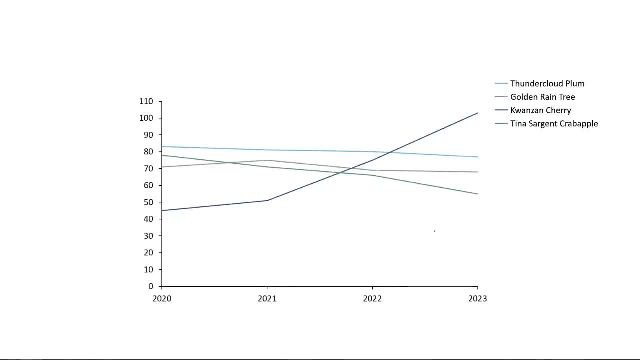 line chart and the message changes entirely. Here you can kind of see this Kwanzaan cherry data increasing over time. So the message might be something like: amidst lackluster sales for most tree species, sales of Kwanzaan cherry have grown steadily since 2020.. You. 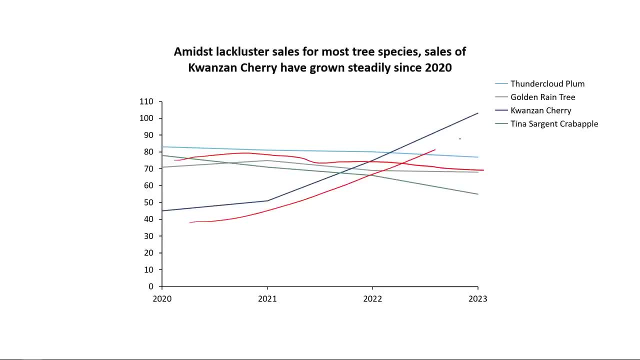 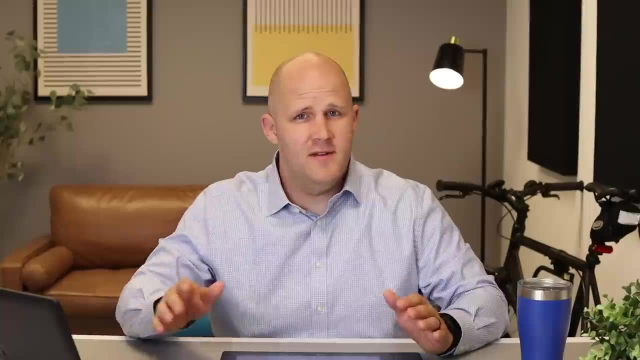 can kind of see. these other trees are flat to declining, but this one is growing Again. this is all the same data for each one of these charts, but the message is changing ever so subtly. So in the first part of this crash course I'm going to cover the five. 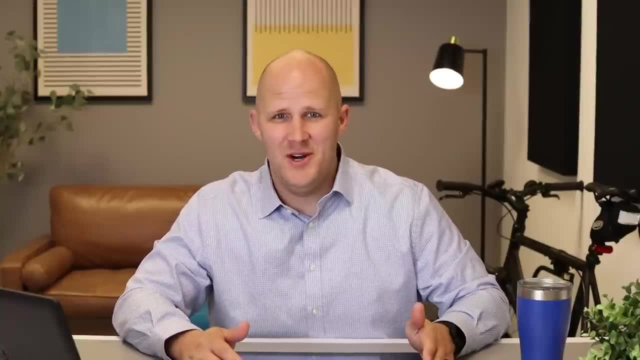 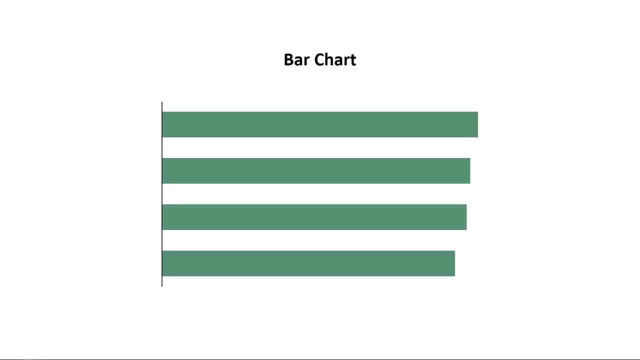 major chart types, starting with the most reliable one, the bar chart. The primary purpose of a bar chart is to compare categories against each other, And this makes sense. You can easily compare the lengths of each of these lines. It's really easy to see which one is. 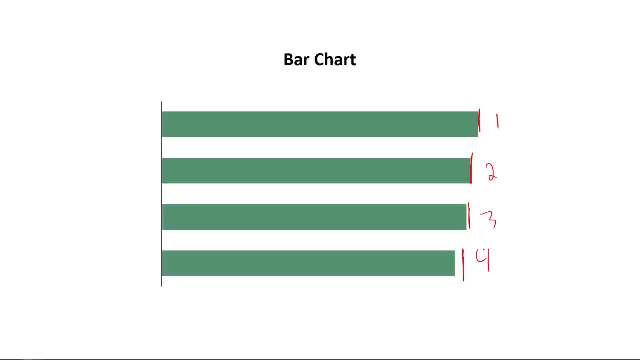 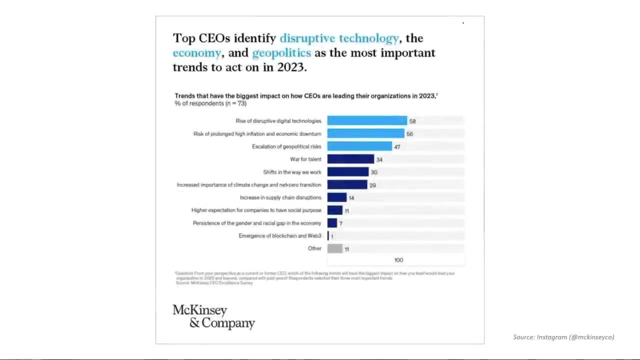 longest, second longest, and so on. It's easy to read, it's precise and it's incredibly reliable. Let's take a look at this example from McKinsey. Title says: top CEOs identified disruptive technology, the economy and geopolitics as the most important trends to act on in 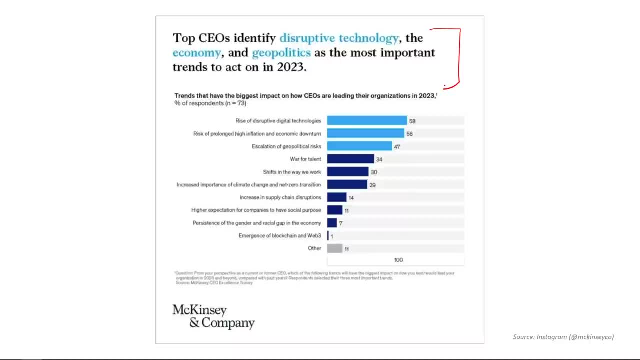 2023.. So what this is showing is survey results about the trends leading into 2023. And with a bar chart, it's really easy to see which one of these is longest, second longest, and so on. So what they've done is they've highlighted these top three bars right here. These are: 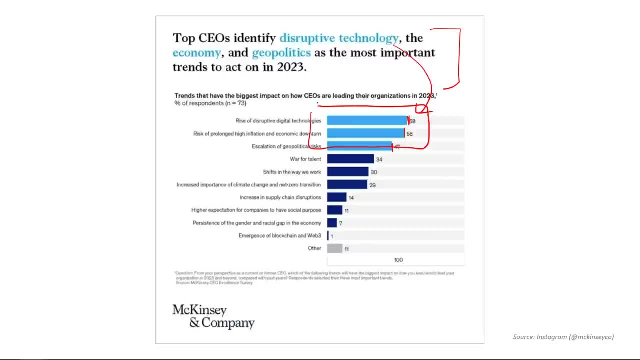 the most important. It's clear, it's interesting and it communicates the message really effectively. And that's what a bar chart is meant for. Again, you want to compare different categories against each other, in this case these different trends. That way, you can easily see which. 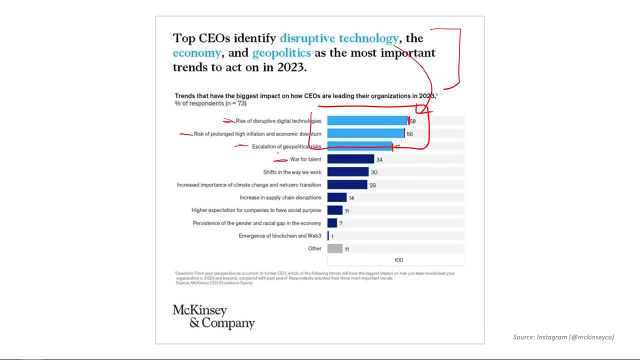 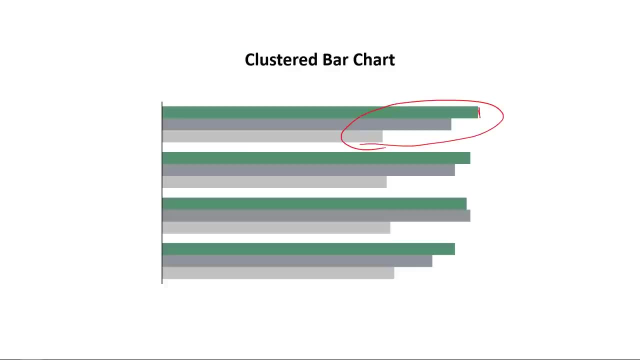 one is the highest or has the biggest value or what have you. And of course there's a few different variations to the bar chart. There's a clustered bar chart which kind of focuses on these subcategories. right here You can compare this: green, dark, gray, light. 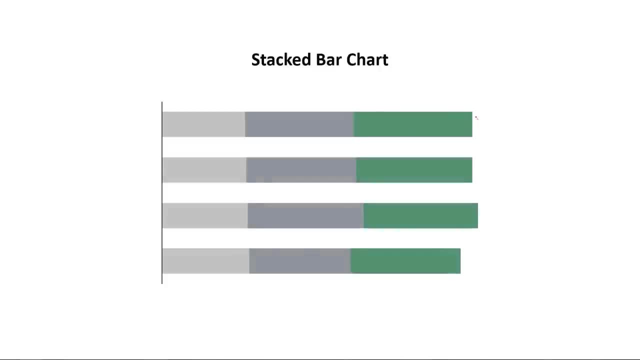 gray against each other. There's the stacked bar chart, which focuses on the overall size of these different subcategories put together, while still being able to show the relative differences of each of the subcategories. stacked bar chart, where all the bars are the same length but the subcategories differ from. 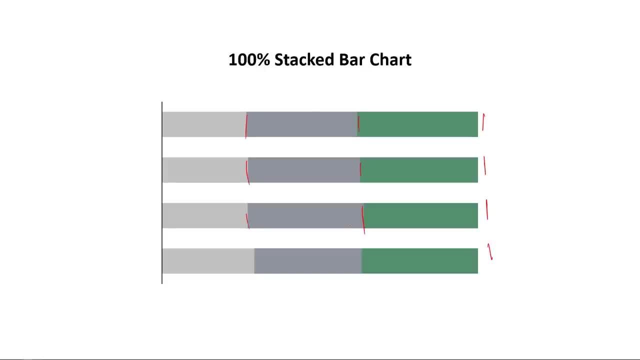 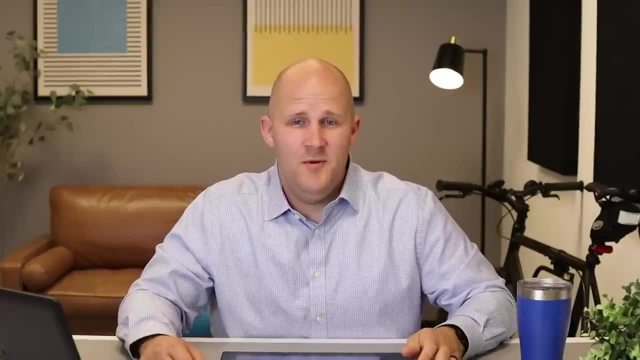 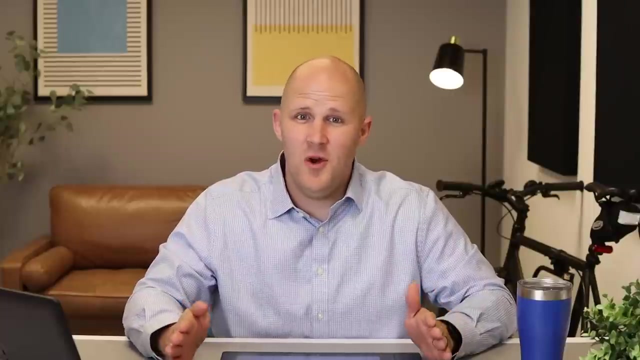 category to category so you can see kind of the relative changes. when you're trying to decide between these different variations, the question you should be asking yourself is: what's easiest to compare. with a clustered bar chart, it's really easy to compare the different subcategories against each other. versus a stacked bar chart, it's easy to compare the overall totals of all. 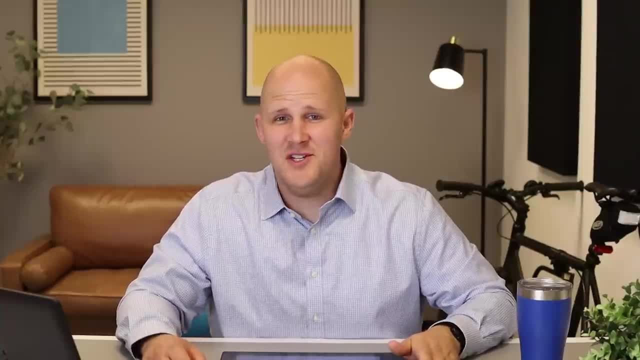 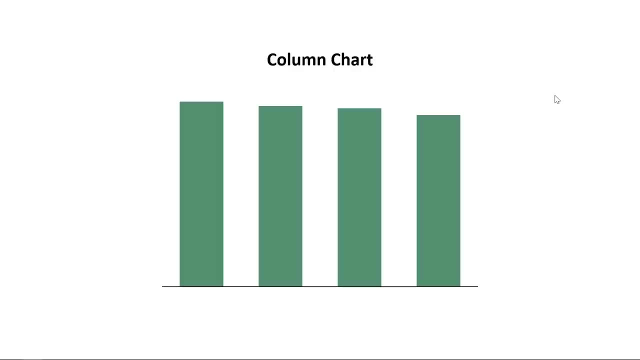 the subcategories put together. but the most important thing to remember with a bar chart is that it's easy for comparing categories against each other. the next chart on our list is a column chart, and this one's really similar to a bar chart, and that it's easy to compare these. 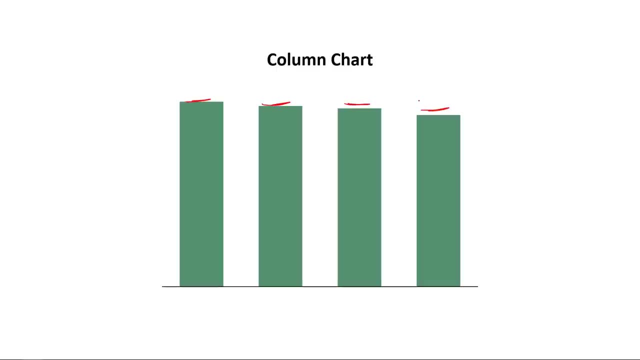 different categories against each other, but there are a few reasons why you'd want to use a column chart over a bar chart, and vice versa. the primary reason is that column charts are good for change over time. that's because our brains naturally read these charts from left to right. take a look at. 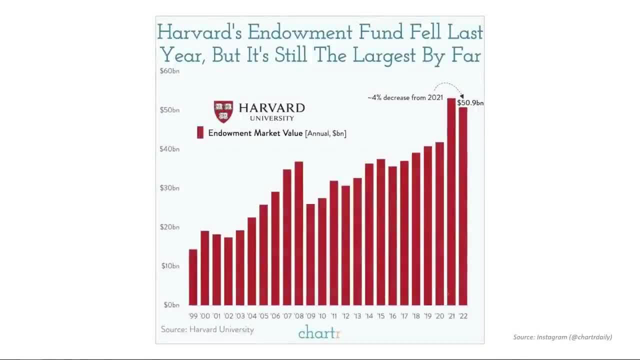 this example from charter. it shows the changes in harvard's endowment fund by year and year, starting from 99 all the way up through 2022, and the natural tendency with this kind of chart is to read it from left to right. so a column chart makes sense, whereas a bar chart might be a little. 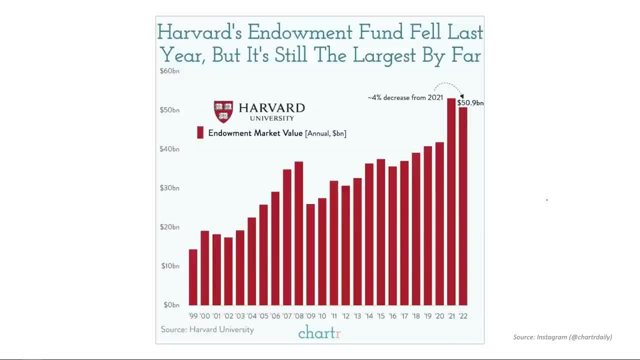 bit more difficult if it was from top to bottom. notice how, with this chart, though, the focus is still on the individual columns and comparing them against each other. this says four percent decrease from 2021. it's comparing the total for 2021 to 2022, emphasized with this arrow. 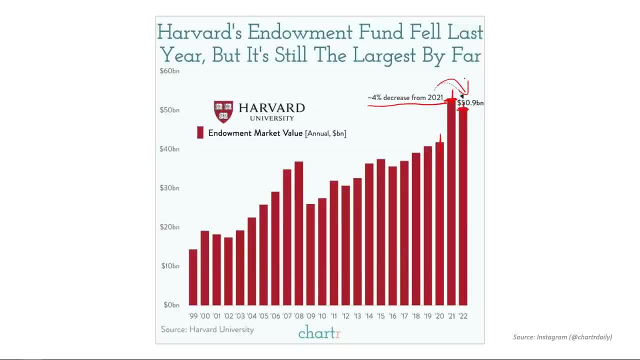 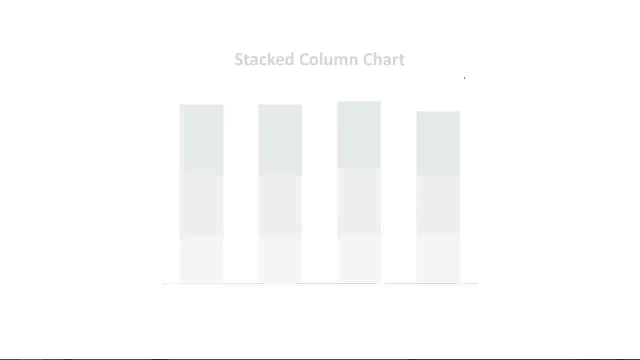 right here. so for this message, a column chart is a really good choice. with a column chart you have the same variations that you have with a bar chart. you've got the clustered column chart, stacked column chart and, of course, the 100 stacked column chart. and again the question you want to. 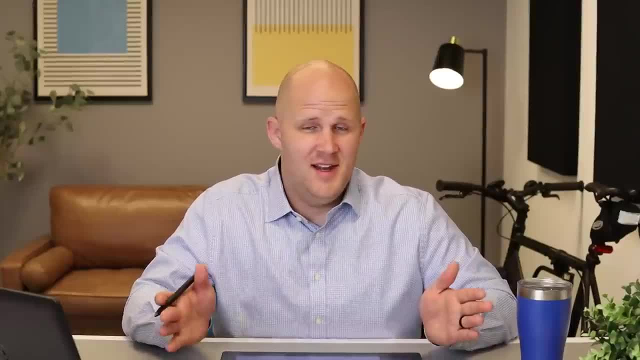 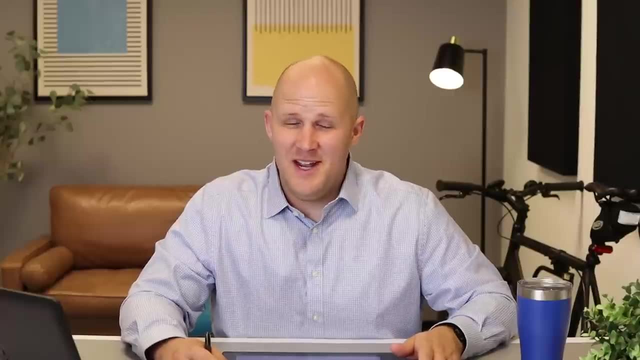 ask yourself is what's easiest to compare with each of these charts? are you comparing subcategories, the category totals or maybe the subtle changes in categories over time? the next chart i'm going to cover is a pie chart, and this is by far the most controversial chart in the data vision. 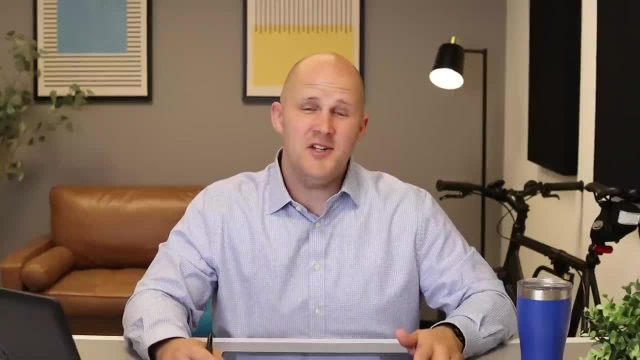 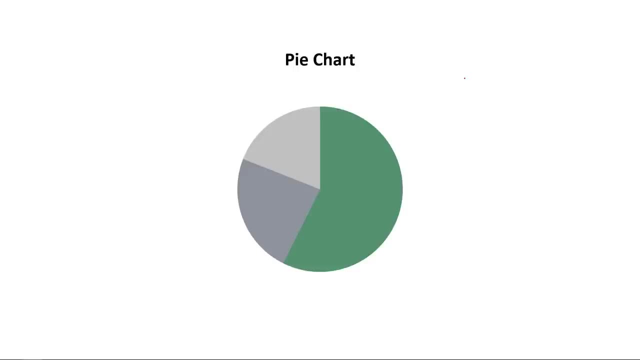 ization world, and there's good reason for that. but the truth is, the pie chart does have its place when it's used correctly, unlike a bar or column chart. you don't want to use a pie chart to compare categories against each other. the primary purpose of a pie chart is to compare a value against the. 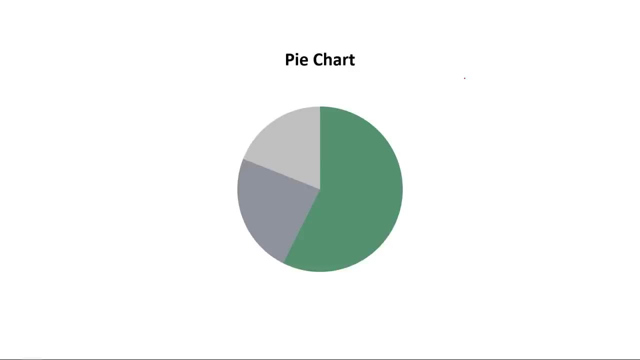 total or compare multiple values against the total. so in practical terms, what this means is you're taking one slice and comparing it to the total of the entire pie, and the shape of the pie chart really lends to this, because our brains kind of naturally associate circles with 100. so it's not 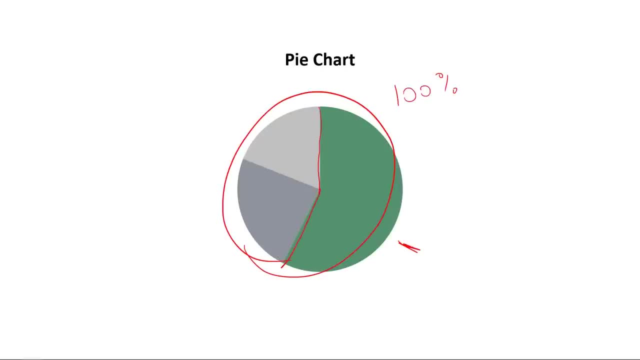 that hard for our brains to take a slice of this and guess roughly what the percentage of it is. so maybe this is 55, for example. where people mostly go wrong is when they try to compare the size of these different slices against each other- this one versus this one versus this one, because that's. 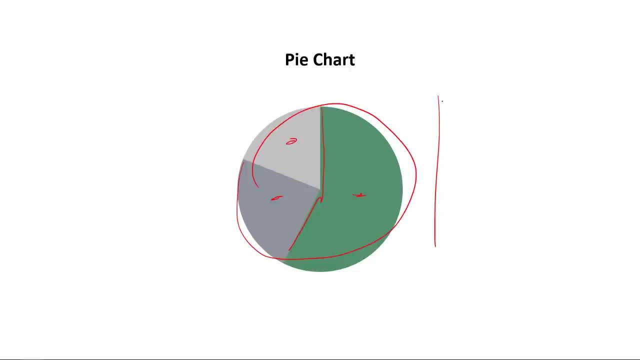 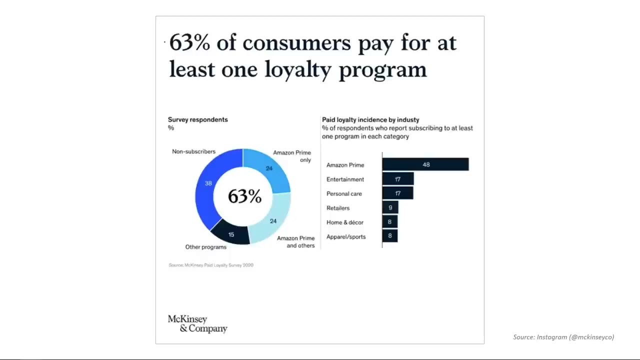 pretty hard to do. you'd be much better off with a bar chart. let's take a look at this mckinsey example. the title says 63 of consumers pay for at least one loyalty program and here you have a donut chart which is basically like a pie chart, but with this kind of center taken out. what it's? 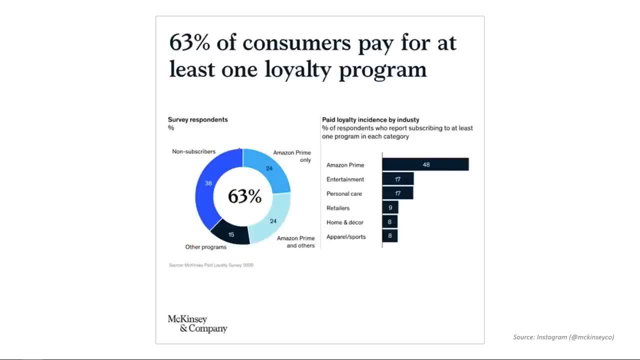 saying is: 63 of consumers pay for at least one of these three loyalty programs, or i guess, amazon prime, amazon prime, and i don't know what they're doing, but they're paying for at least one loyalty program. and here you have a donut chart which is basically like a pie chart, but with this kind of 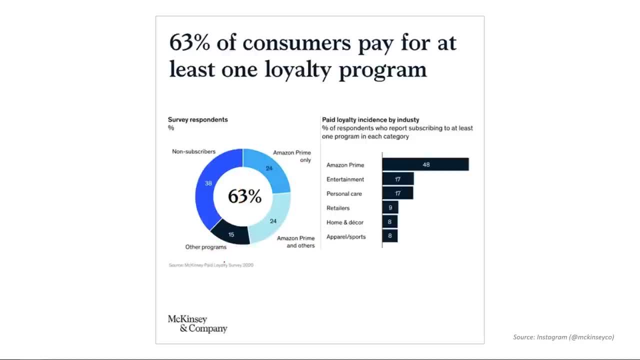 and others, or just other programs, and what it's trying to emphasize with this title is this section right here. in other words, it's saying 63 of people either have amazon prime, only amazon prime and other loyalty programs or just other loyalty programs, and this would be a little bit more. 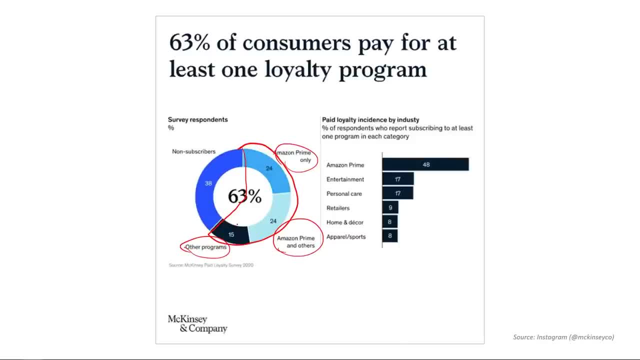 difficult to show in a bar or a column chart, or any other chart for that matter. so in this specific case, a pie chart or a donut chart works really well, but if the message were slightly different. let's say, the percentage of non-subscribers is greater than the percentage of subscribers. 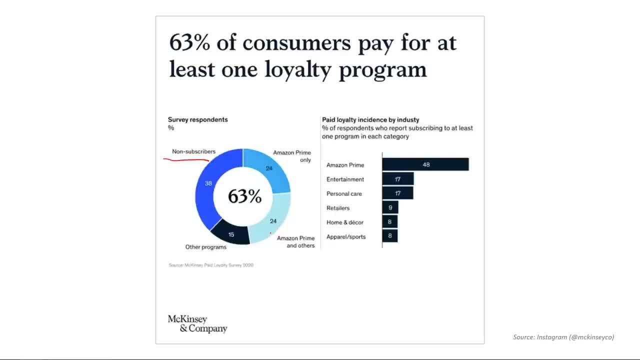 then this message wouldn't come through quite as clearly. instead, you'd be better off with a bar chart. the reason for that is it's really easy to compare the lengths of these different bars. so this would be non-subscribers, and this would be subscribers just like with the other chart. there are some variations to this chart. 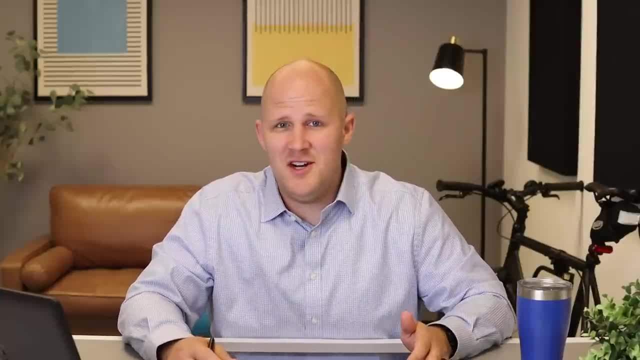 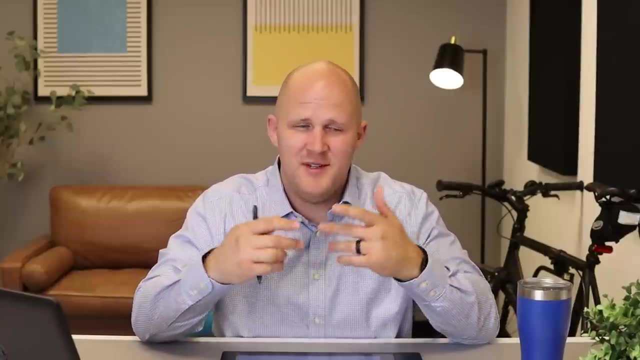 one we just saw which is a donut chart, which is essentially the same as a pie chart, but with no hole, so you can put extra data in there. the only downside to a donut chart is it's harder to see the internal angles, which for some people can make. 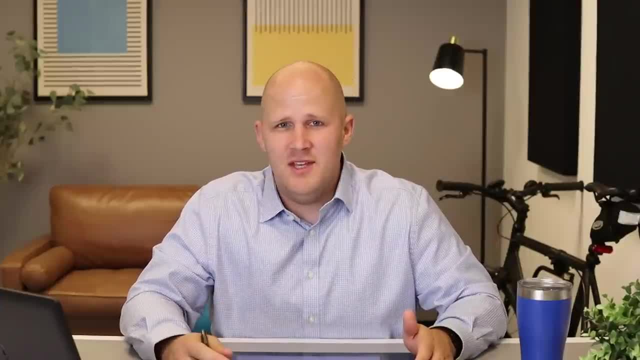 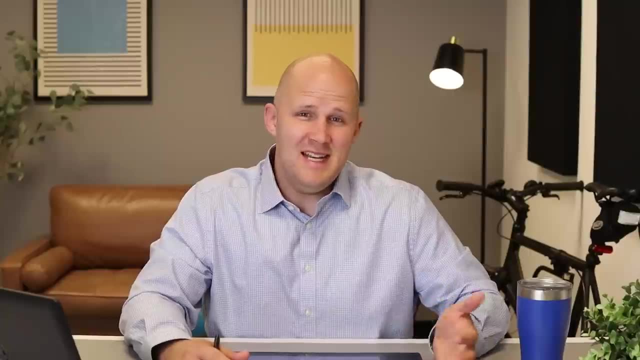 things just a little bit difficult, but for the most part they're very commonly used and a good chart choice. there are some other variations, like a sunburst chart or a tree map, which follow the same idea as a pie chart, but look just a little bit differently. the next chart on our list is a. 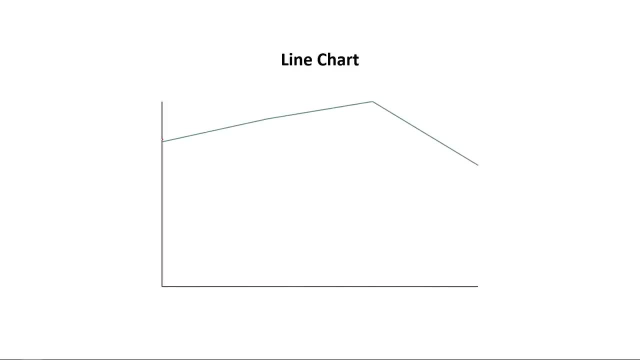 line chart, and this is good for showing changes or trends or patterns over time. it's very similar to a column chart, but the difference is, instead of focusing on each individual column, all the points are connected together, so you kind of focus on the data as a whole. this helps emphasize things. 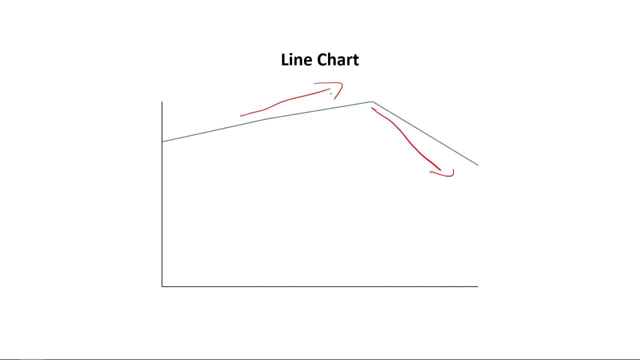 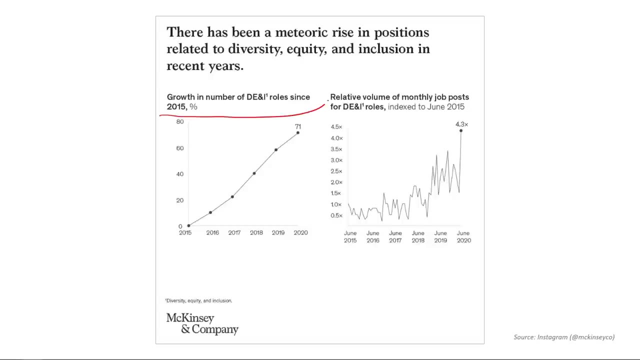 like downward trends or spikes, upward trends, anomalies in the data, things like that. so, for example, here we have a chart about the growth in the number of diversity, equity and inclusion roles since 2015.. and if you take a look at the message here, it's talking about a meteoric rise. 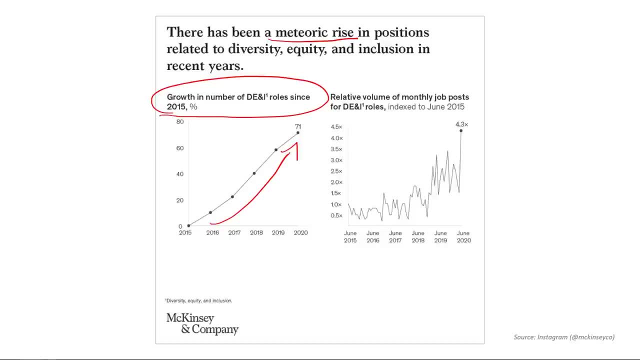 so a line chart is good for this because, a- it's expressed over time, but then b, it's showing this like strong upward trend. yes, you could still see that data in a column chart, but it gets emphasized just a little bit more in a line chart because you have these: 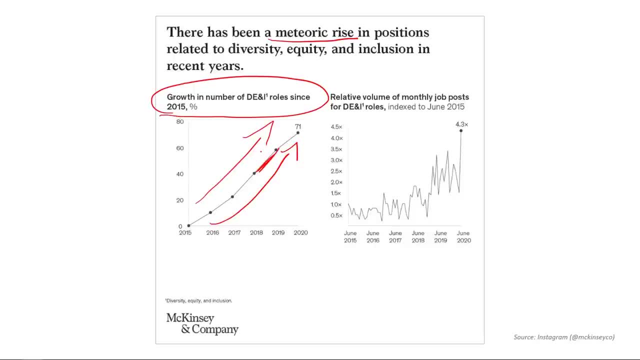 sloping lines. the caution with line charts is you want to make sure that you're using them for data that has a natural order to it. so, for example, time has a natural order, but let's say you had different categories. if there's no natural order to this data, you can put. 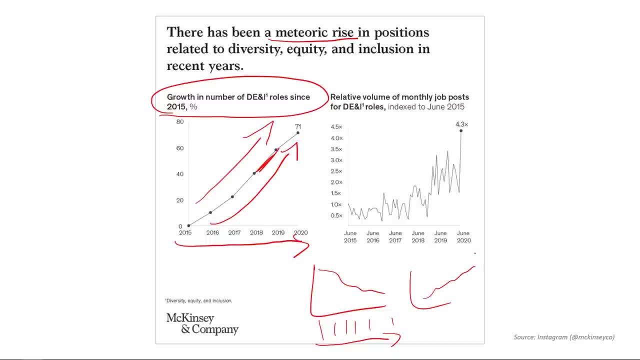 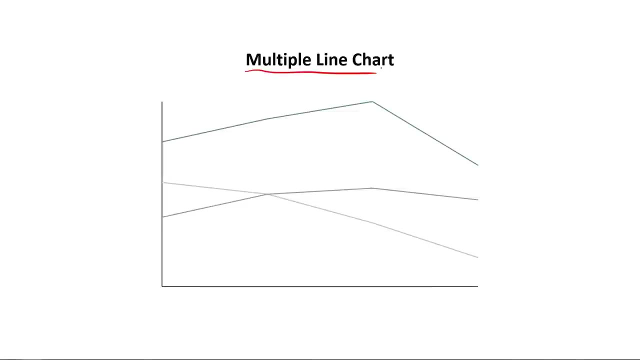 it in any order you want, and you could be showing a trend that doesn't necessarily exist, So be careful to use this for data that's expressed over time or in some other natural order. There's a few different common variations to a line chart. One of them, of course, is to just put multiple lines. 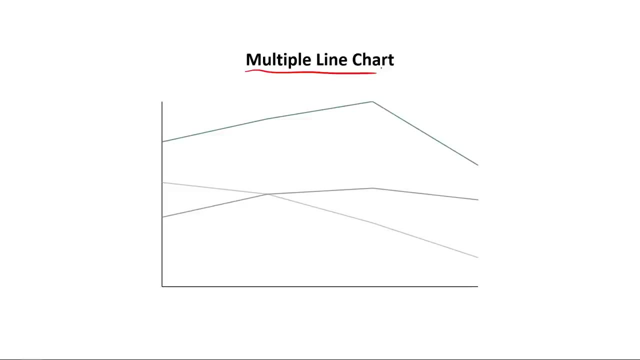 on the chart. This is good for a few different things. One thing is emphasizing how one of the lines is different than the other, but sometimes you can also have a chart where you're trying to show that all the lines kind of follow the same pattern. Another variation to the line chart is an 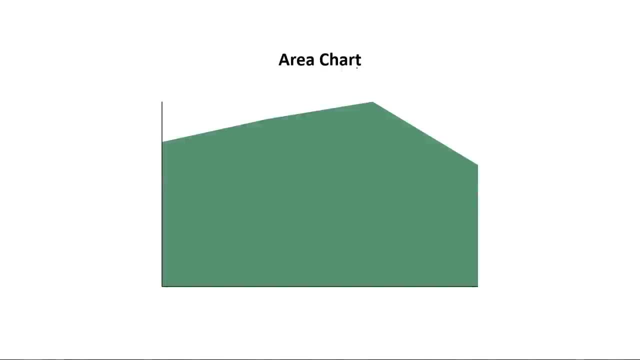 area chart. Now we go into a lot more detail on this chart in the course, but basically you can think of it as a column chart combined with a line chart. Whereas a column chart kind of focuses on these as values and a line chart focuses on the overall trend, an area chart does a little bit of. 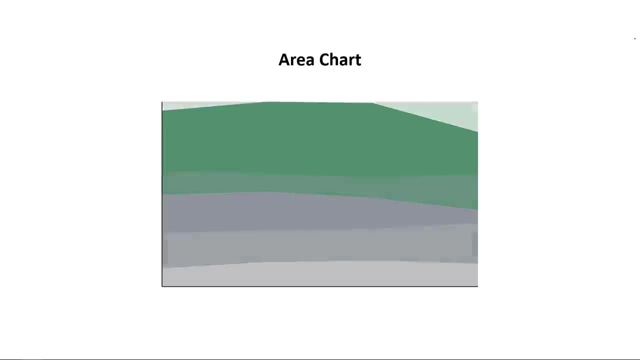 both. Then, of course, you have a stacked area chart and a 100% stacked area chart, which again serve much of the same function As a 100% stacked column chart, where it focuses on how these, how the makeup of these different categories changes over time. The next chart on our list is a scatter plot, and this is one of my. 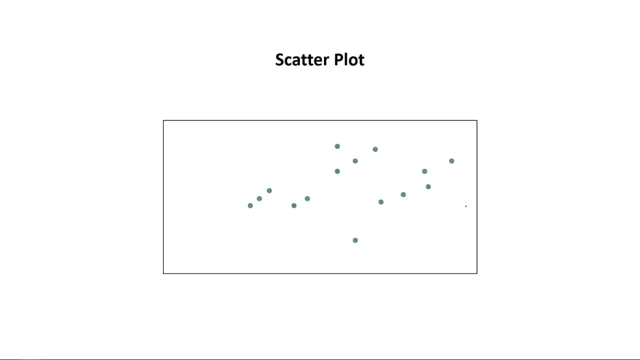 favorite charts. The primary purpose of a scatter plot is to show the relationship between two variables. So imagine, for example, if this represented weight in this represented height. generally speaking, the taller someone gets, the more they tend to weigh. And this is represented mathematically with the coefficient of determination, or r squared. 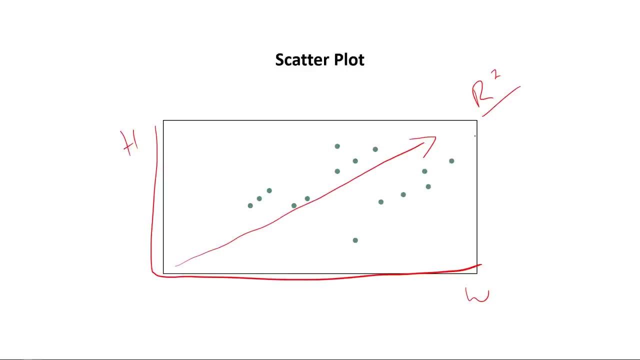 So with a scatter plot, you could be showing a few different things. you could be showing positive correlation, you could be showing negative correlation or you could be showing no correlation at all, which in itself can be telling Sometimes. it's also good for highlighting. 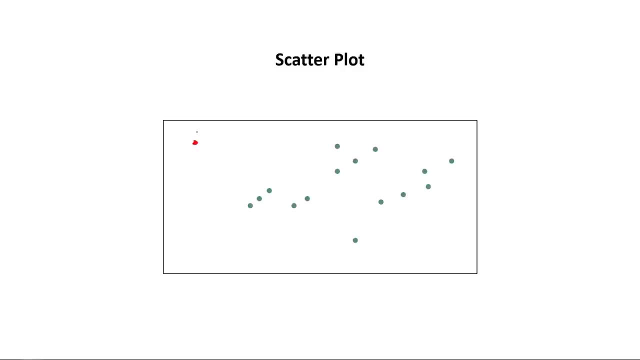 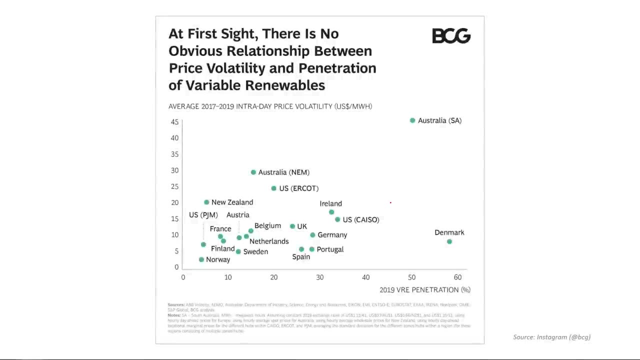 outliers. So, for example, if you had a dot way over here that you wanted to emphasize, or it's good for just showing where a specific dot falls on this plot, Here's a pretty good example from BCG. what it's showing is price volatility. 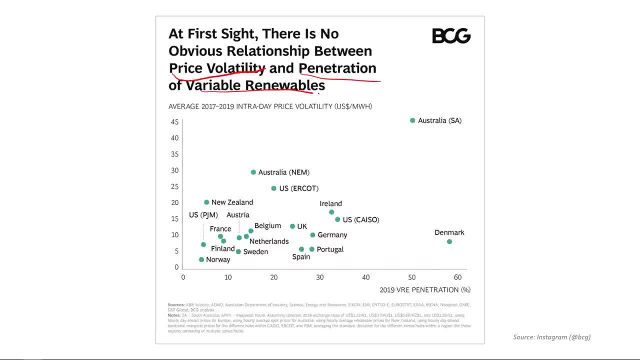 versus this VRE, or penetration of variable renewables, And what it's trying to communicate, this chart, actually, is that they don't believe there's much of a correlation at all, which, like I said, in itself can be telling. The other powerful thing about scatter plots is, you can add, 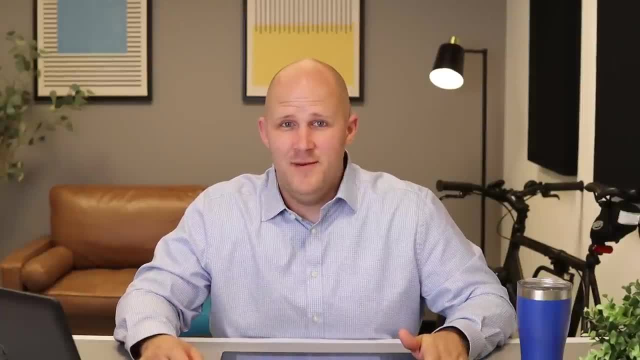 additional variables to make the information a little bit more rich. So, for example, if you wanted to change the size of each of these data points, for example, if you wanted to change every point size of each of the dots, if you wanted them to represent something else, then voila you have a. 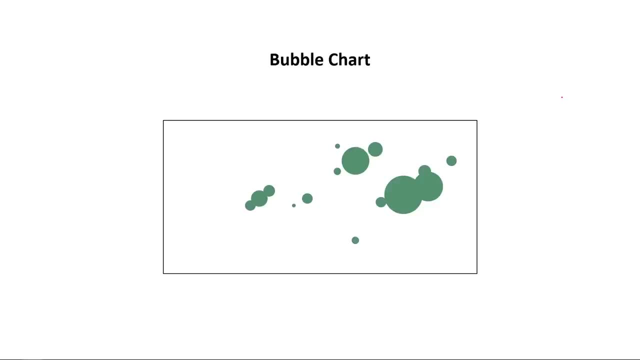 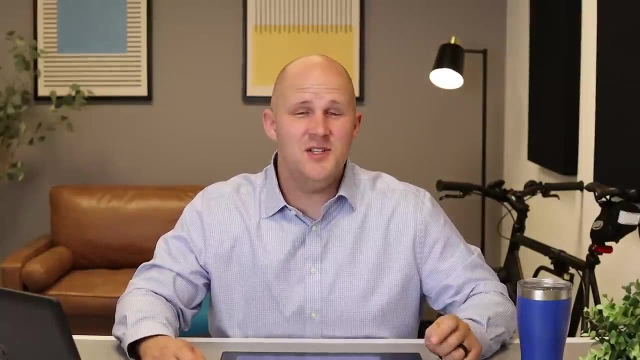 bubble chart and again you have that much more information to communicate to the audience. you could also change the color of the dots, or you can even change the symbols themselves. however, i would really caution against this, unless you absolutely have to. the temptation with scatter plots is to 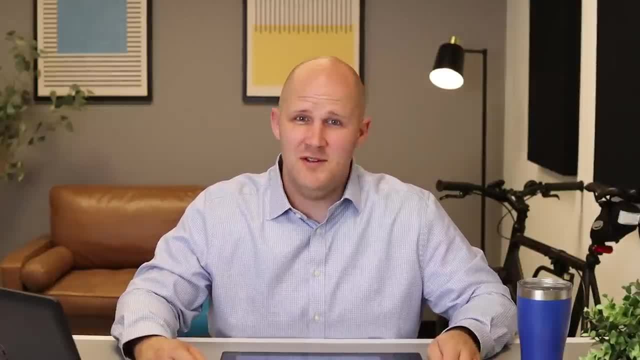 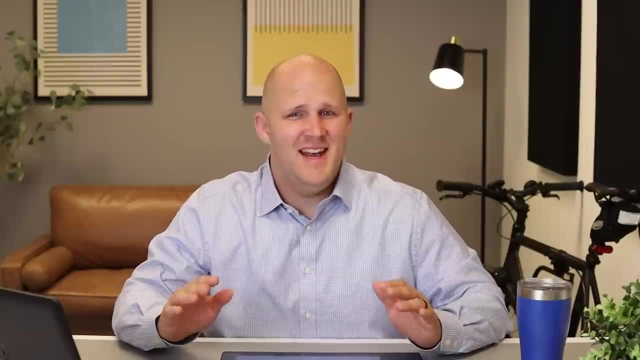 introduce all these extra variables. it just makes it more confusing for your audience. focus on your main message and make sure that comes through clearly in your chart. so, when it comes to effective data visualization, 90 of the time you're going to be able to use one of the five charts we just 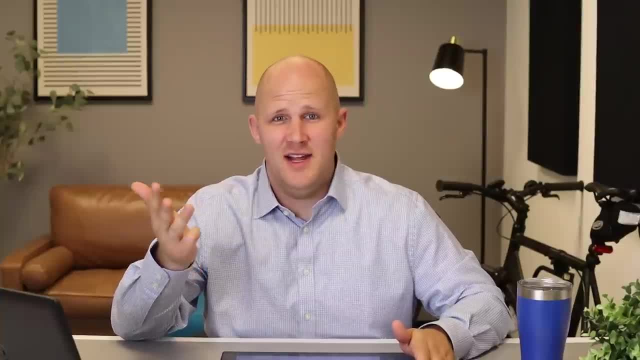 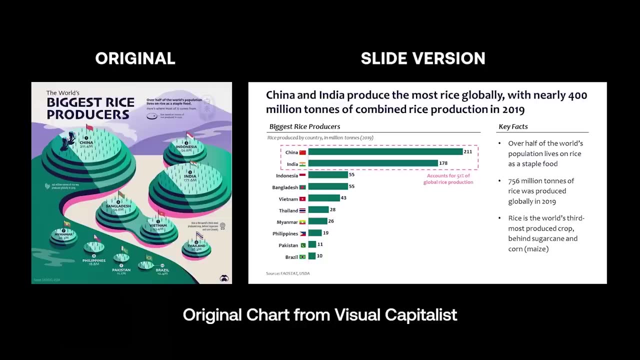 went over bar chart, column chart, pie chart, line chart and scatter plot. in a recent video, i remade fancy charts into realistic slides and in every single case i used one of these charts, and in other videos i follow the same pattern. so the key to good data visualization is learning when to use. 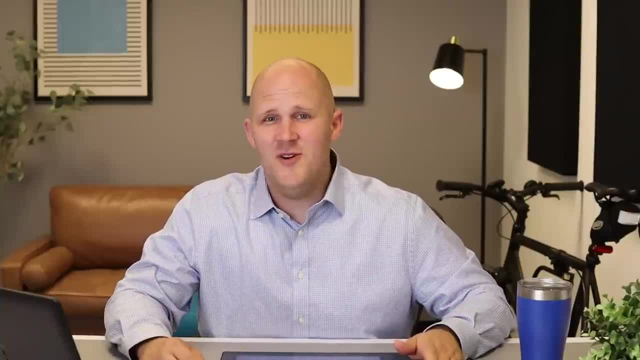 these charts and learning it really, really well. the best way to do that, of course, is with practice and repetition, but i promise you, if you can focus on this core set of skills, you're going to be able to use it in a lot of ways, and i'm going to show you how to do that. 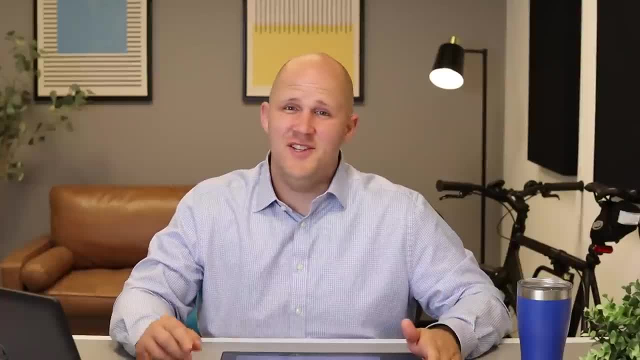 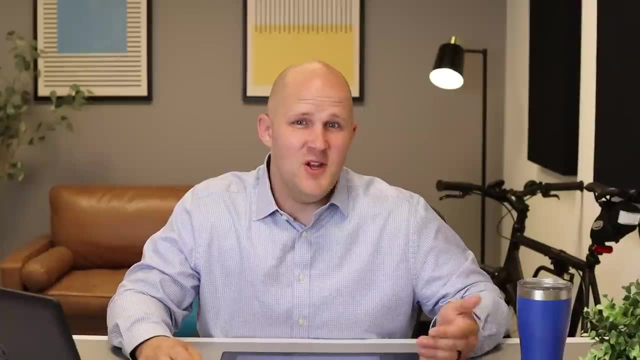 you'll get really, really good at data visualization. once again, if you're interested in this sort of topic, make sure you check out our course over at theanalystacademycom. we go in much greater detail and really explain the nuances of each of the different chart types, and it's complete with 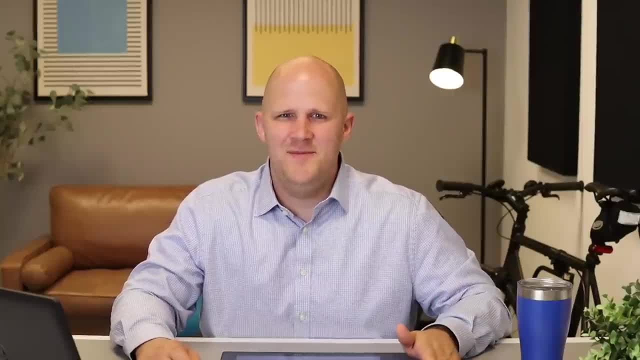 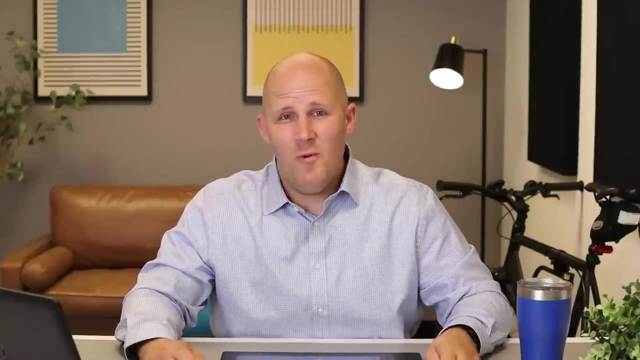 examples, exercises, quizzes, that sort of thing, so make sure you check it out. in addition to these core chart types, there are additional ways to visualize your data, and we don't have time to get into all of them now, but one in particular that i want to talk about is tables. tables can. 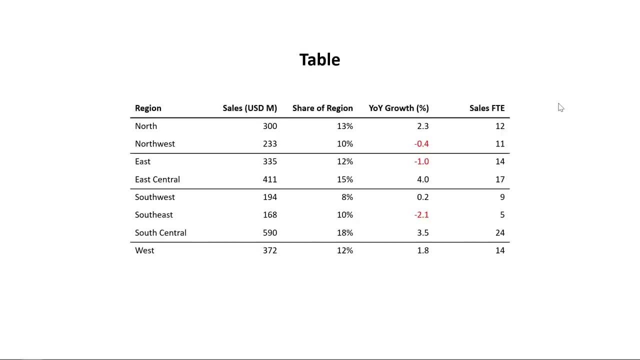 be especially good for two reasons. the first is when you need to show precise values. so, for example, here we have a basic table that shows sales for different regions and a few additional metrics like share growth and the number of full-time employees, and a table would be really good here if i wanted to show specific. 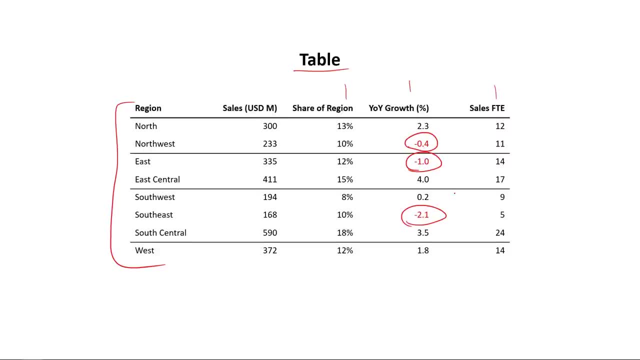 values like the negative growth values, for example. for example, if my message was in the east region, we saw negative one percent growth year over year, then this would be a good choice, because i'm calling out a specific value for each of the different regions, so i'm going to call out a. 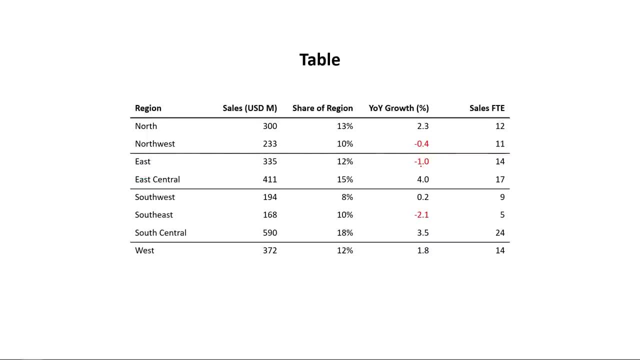 specific data point. the other major reason is, if you're trying to show multiple types of data in the same space, here we're not just showing sales, but we're also showing the share, growth and number full-time employees, and that would be pretty difficult to display in a chart. is it possible? 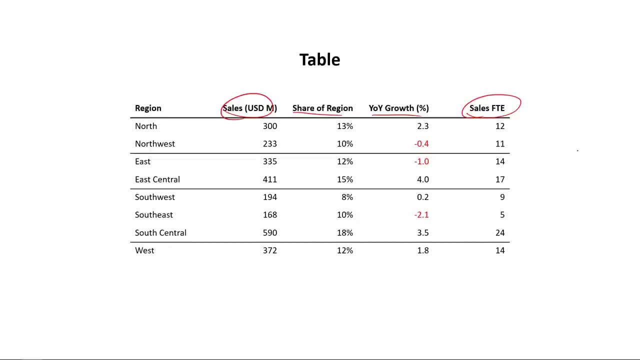 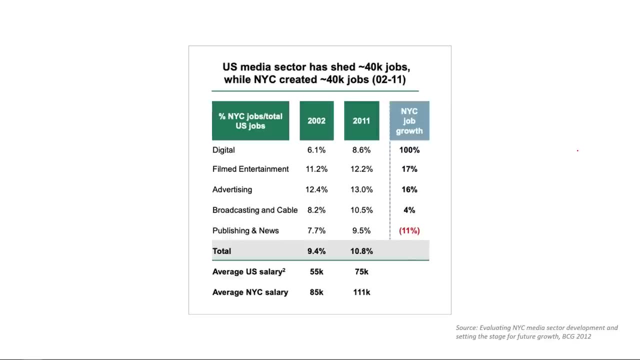 yes, but it would just make things a little bit more confusing. there's a good example of this by bcg. so here's a chart from a presentation about the new york media sector, and what it's primarily showing is the percentage of new york jobs versus total jobs. 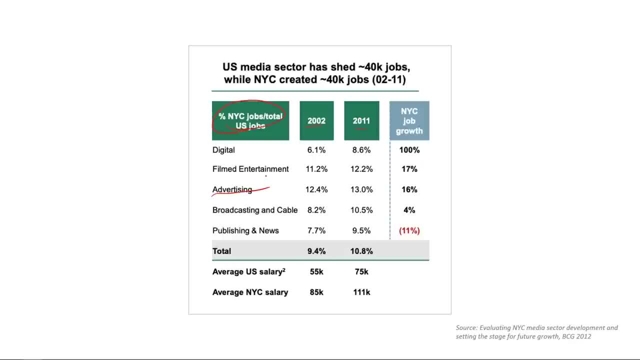 in each of these different years. so, for example, in advertising, 12 of the jobs were in new york versus the rest of the us, and then in 2011 that jumped to 13. so if these individual values themselves are important, then a table is a good choice here. but the primary reason to use a table 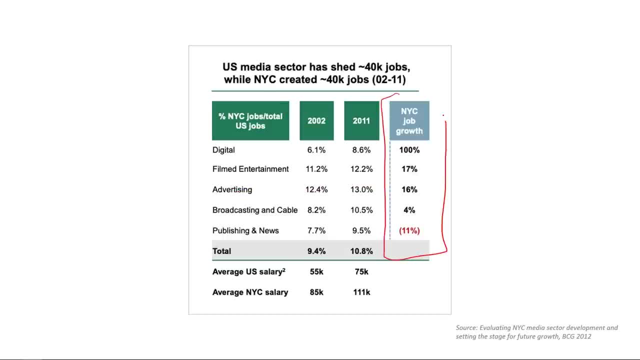 here is because you're also showing this extra information. for example, the growth in new york city jobs. these are both percentages, but they're showing fundamentally different data. plus, you have these numbers down here where you're showing absolute values. these are salary numbers. trying to put all this information in a chart would be difficult and confusing. 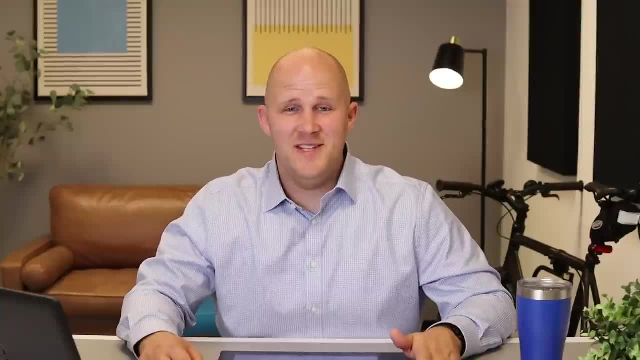 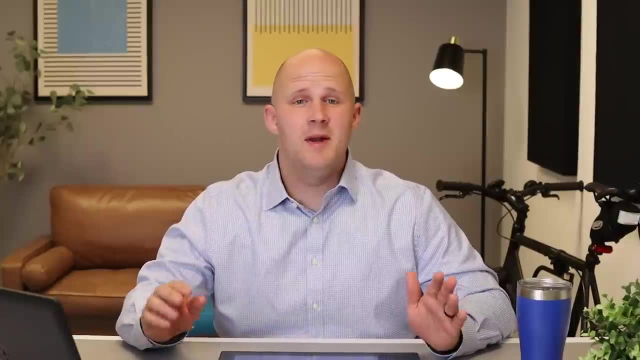 so here the table is a good choice. all right, now that we've talked about the different ways to visualize your data, let's talk about design best practices. now. there's a lot of different things i could talk about here, but i'm going to boil it down into two key ideas. 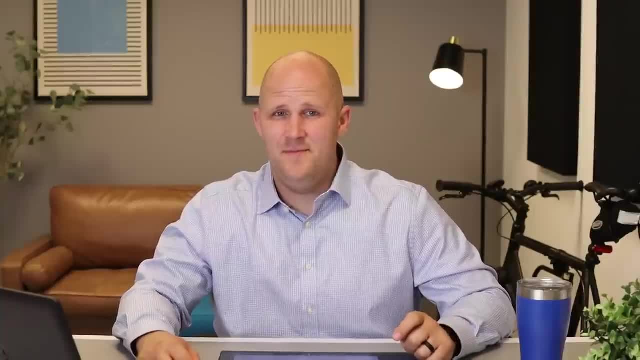 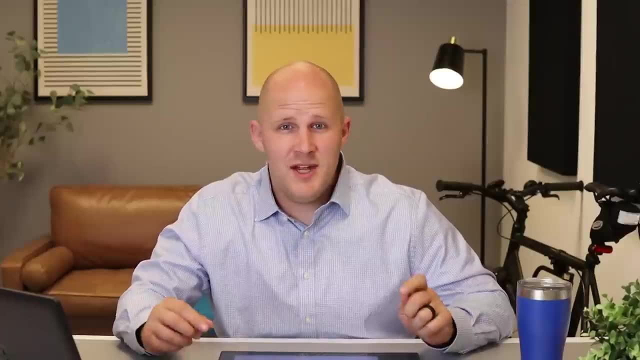 the first is to make sure your message is clear. now this sounds like a pretty basic thing, but you can do this by looking at the chart, and you can also do this by looking at the chart itself, so you can see how many people are really surprised, how many people really messed this up. 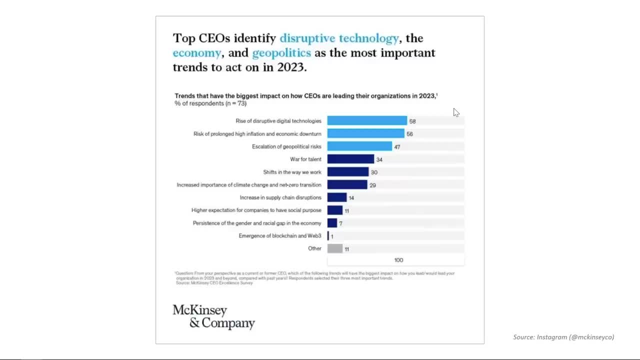 you have an overall message that you want to communicate, make sure that message comes through very clearly in the chart itself, and there's a few different ways you can do that. let's revisit this chart for mckinsey. remember, it's just a simple bar chart comparing these different trends against. 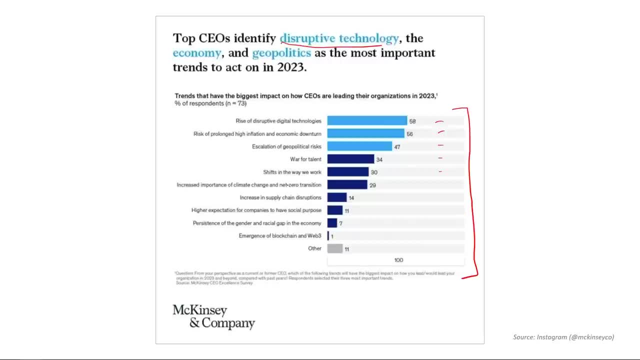 each other, but they do a few different things- to call attention to the message of the chart, which is that these three trends- disruptive technology, economy and geopolitics- and we've heard a lot of them in the last few weeks and you can see that they have a clear title and this is the easiest and most important thing you can do for effective. 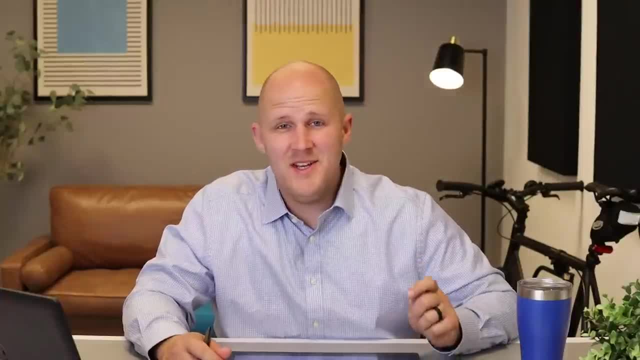 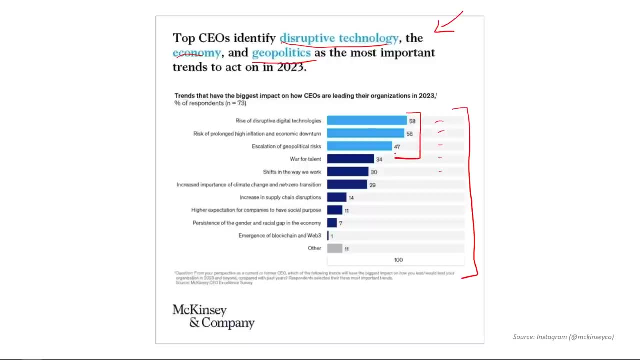 communication have a clear title that explicitly communicates the message you're trying to tell the audience. the other thing they've done is they've highlighted the bars themselves, drawing attention to them as the most important trends, and, of course, they've ranked these trends in order to make it that much easier. these are subtle things, but they have a huge impact in the overall 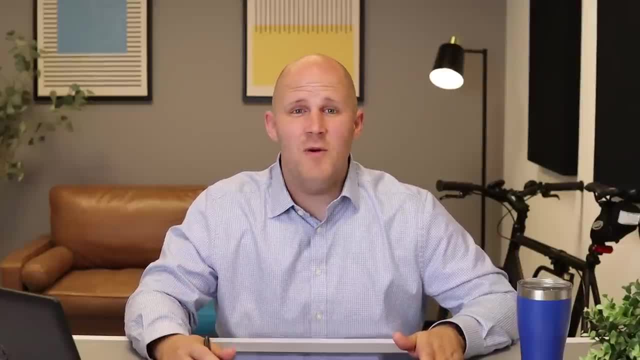 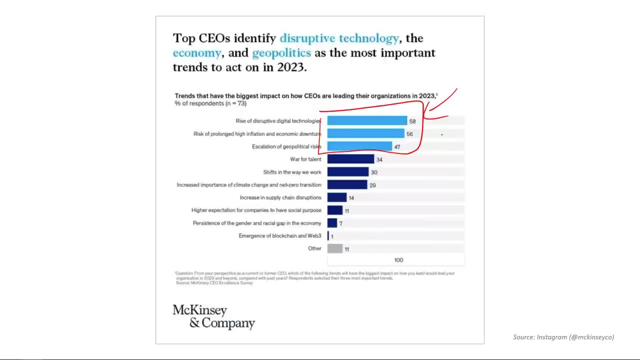 of your message, Figure out what your message is and find a way to communicate that clearly. There are a few other things they could have done. They could have put a box around these bars, maybe an arrow, some additional text right here. All of these are ways you can draw attention to. 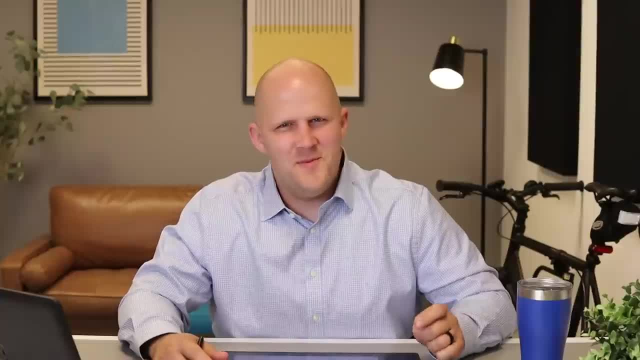 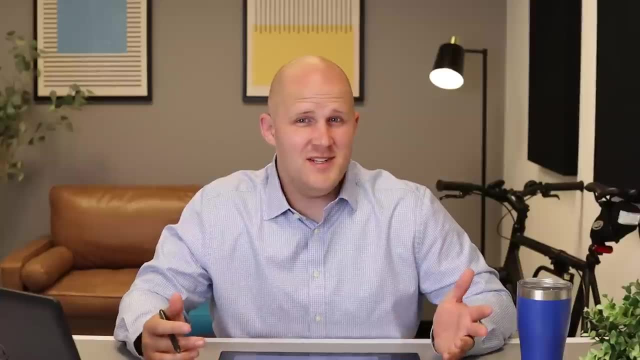 your message, which, again, is really important. Another really important principle of good chart design is removing the clutter from your chart. You'd be surprised how many things you can take away from your chart that really don't matter to the overall message or to the data itself. 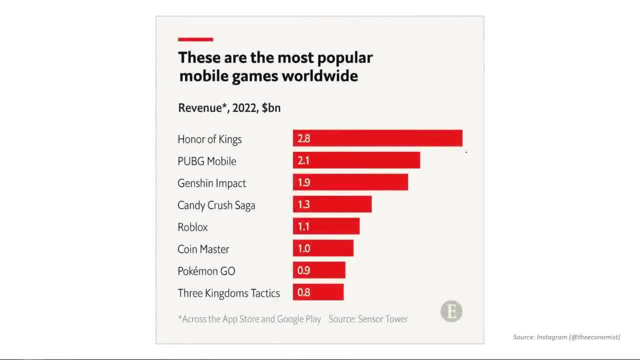 Here's an example from The Economist that highlights this really well. The title itself is really simple. The subtitle and explanation also very simple and clear. But notice how there's not even any axes on this chart. There's no data labels right here to clutter the message. 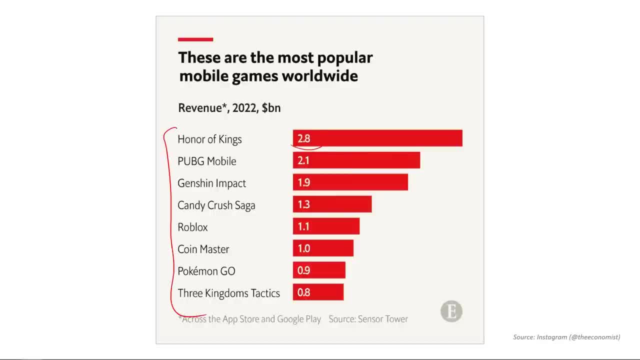 All it is are the categories labels in the bars themselves, And notice also how they only use one color for this chart. All of those things are a deliberate effort to help you focus on the actual data and not on the actual data. So if you're looking at a chart, you're going to 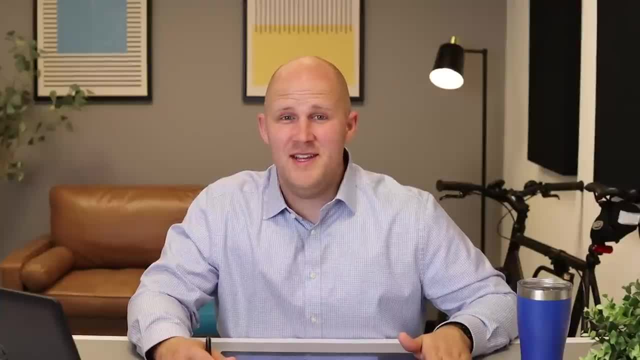 focus on the actual data and not on the actual data. So if you're looking at a chart, you're going to focus on anything else. We actually did a whole video on The Economist and why their charts are so effective. So if you're interested in stuff like that, I'll include a link down in the 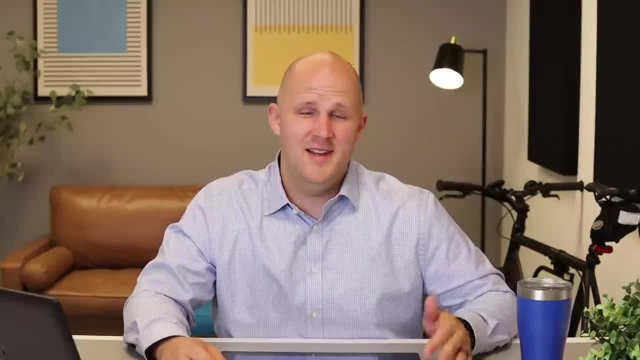 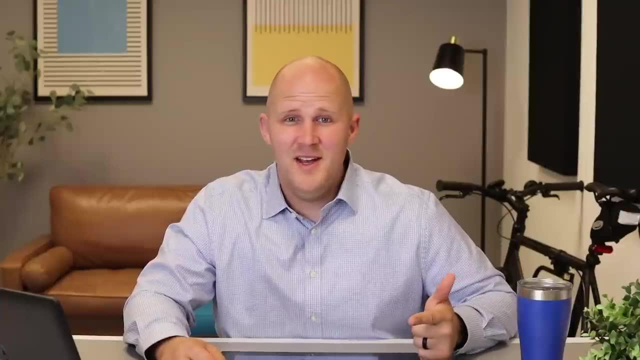 description. So really good chart design comes down to two things: Emphasize your message in the chart and remove the clutter from the chart. And if you can do those two things, and do them really well, your charts are going to look a whole lot better. All right, now that we've 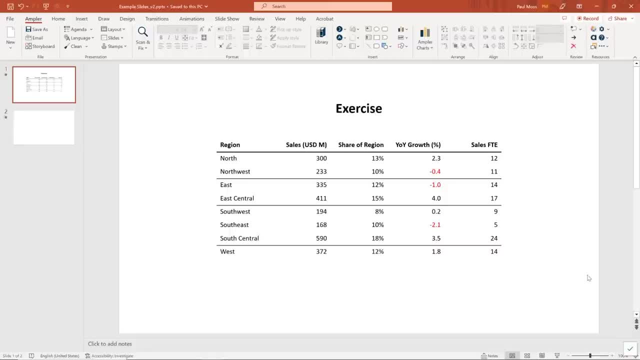 covered the basics. let's walk through an exercise together, All right, so we're going to keep this table example earlier, And all it shows is sales by region, the share of sales for each region, year over year growth and sales FTE. If you want to follow along with this exercise yourself, 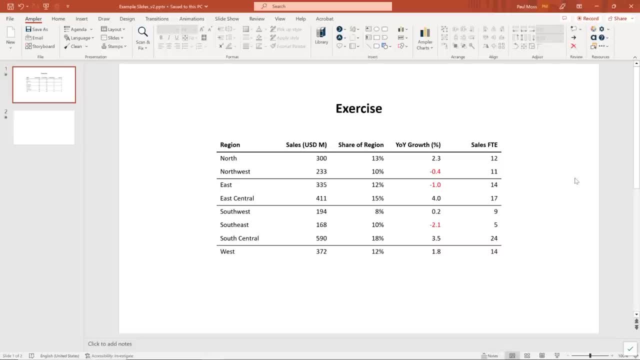 I'll include a download link in the description below, Or, instead of following along, you can do the exercise yourself first and then come back and see the solution here on the video. So let's say your manager says, hey, I want you to help me understand the relationship between overall sales. 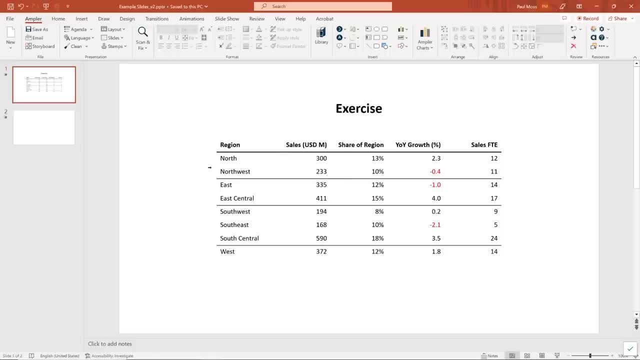 for each region and the share of sales for each region. And if you want to follow along with this exercise yourself, I'll include a download link in the description below. All right, so we have our data here. we just need to figure out which chart type is going to be best for emphasizing that. 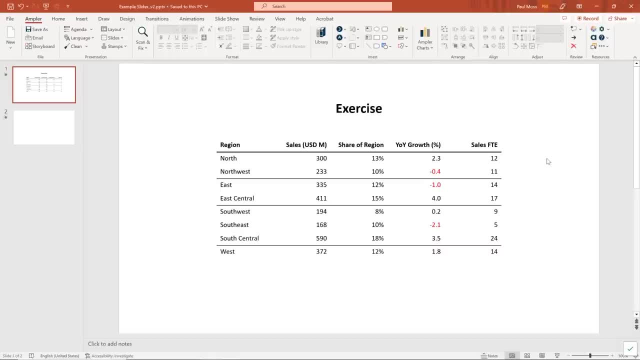 message Going through each of the different chart types. First you have a bar chart. A bar chart would be good for comparing these different categories against each other, But that's not necessarily what we're doing. For example, we're not trying to say that sales in the north is. 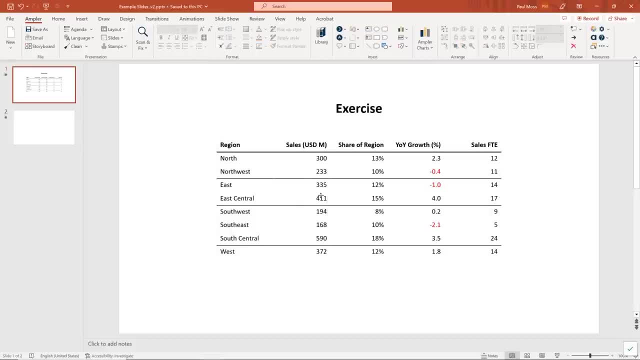 greater than sales in the southeast, or that east central or, excuse me, south central has greater sales than all of them. A bar chart would be great for that, But that's not what we're doing. Likewise a column chart. we're not comparing these against each other And we're not doing it. 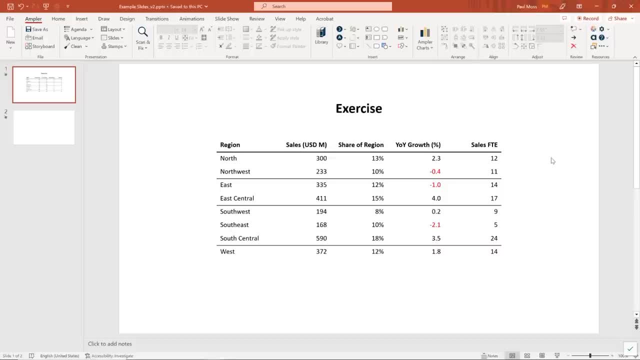 over time. So column chart doesn't really work either. Same thing with a line chart. we're not really trying to show the trend of any particular set of data, We're trying to show the relationship between these two sets of data. So line chart is out also. A pie chart would be good, for example. 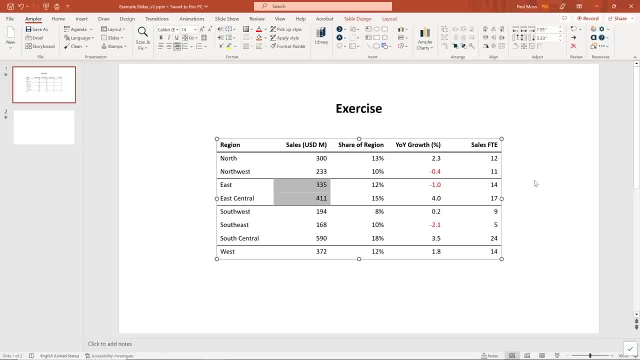 if we were trying to say that east and east central account for a certain percentage of the overall sales. But that's not what we're trying to show. Again, we're trying to show the relationship between these two variables. So, as you might have guessed, a scatterplot is going to be a good choice here. All right, 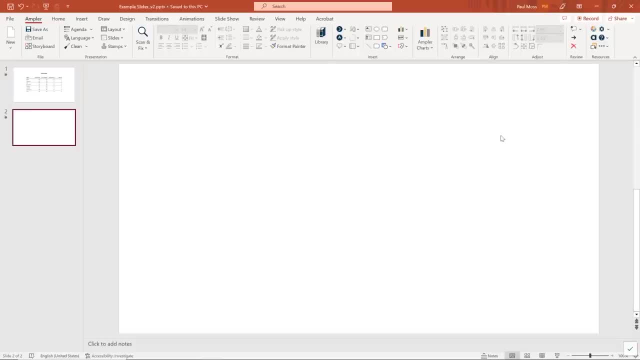 so let's put this data into a scatterplot and see what it shows us. By the way, for this exercise, I'm going to use a tool called Ampler Charts. It's the chart building tool that we use and recommend over at Analyst Academy. It's really robust, lots of excellent functionality And it. 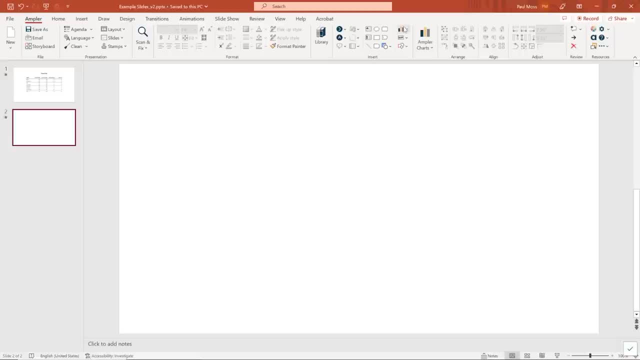 makes chart building really really simple and easy. It's built right into PowerPoint here. you just select the chart that you want. you can customize it really simple and easily, which you're going to see here in a second. But again, it's something we recommend. you can get a free one month trial. 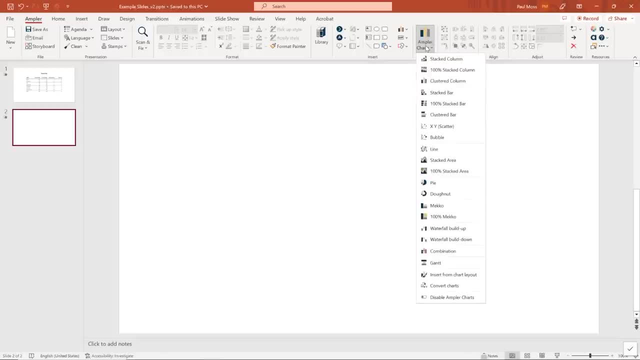 by following the link in the description. All right, so we're going to build a scatterplot, So we'll just go up here, go down to scatter and you can just choose the size. we'll just keep it simple like this. And then just we just need to copy our data into the chart. Oops. 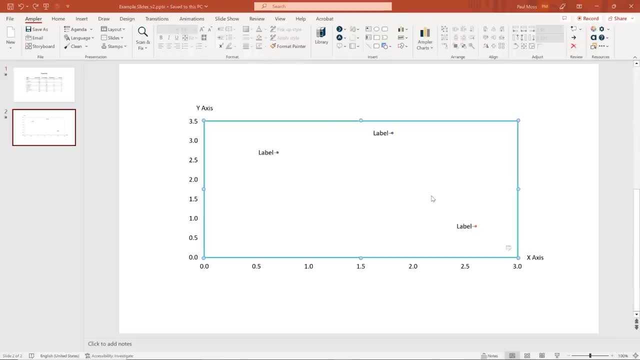 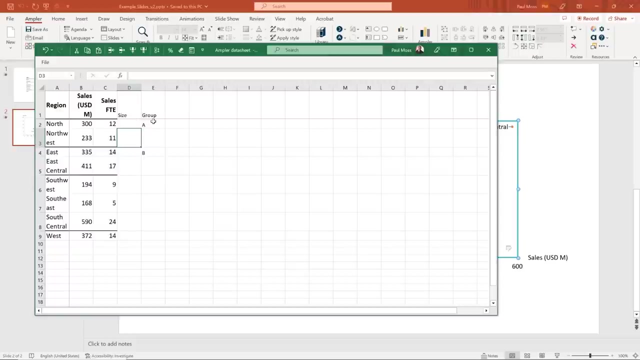 So let's copy this. double click on the chart brings up this Excel like window here And I'll come back over to this one And copy sales FTE. Paste that in here. These two columns are for if you wanted to separate these into different groups. 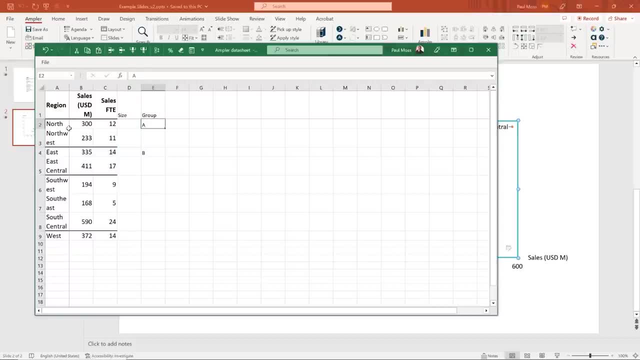 So, for example, if you wanted you know Northwest, East, East, Central North, all to be in a certain group and a certain color, And if you wanted the rest of them to be a different color, that's what you would use this column for, And then you can just copy that into the chart, And then you can. 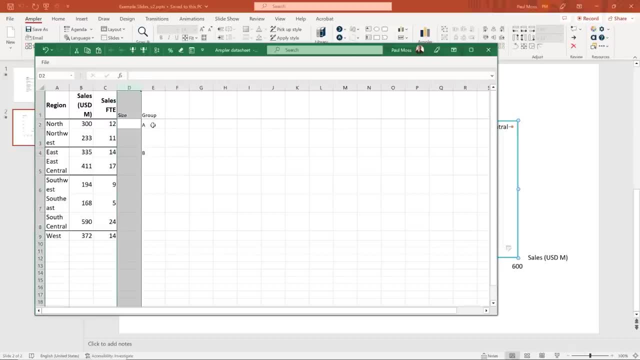 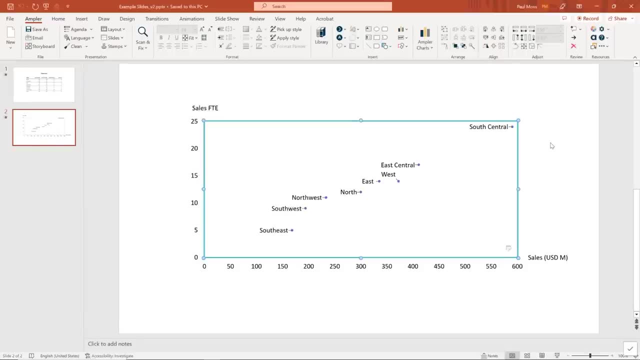 copy that into the chart And then this would be: if you wanted to include an additional variable, turn it into a bubble chart. But we're not going to do either of those things. We're going to keep it simple. So delete those columns And here we go. We already have the data that we're looking for. 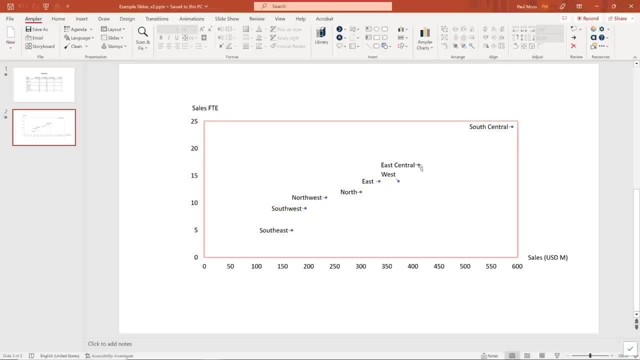 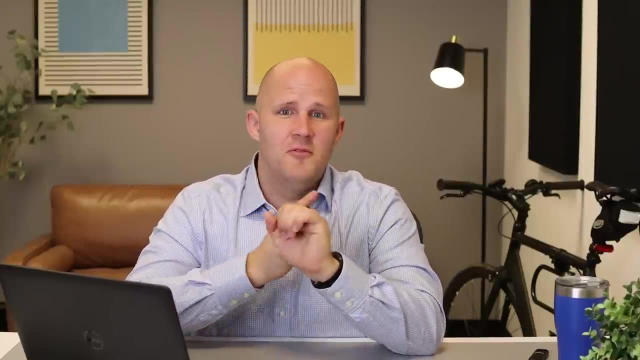 And you can see that there's a general sort of positive correlation here. So when you're trying to build an effective chart, remember there's two things you want to focus on: making sure your message comes through clearly and removing the clutter from your chart. So let's start with the 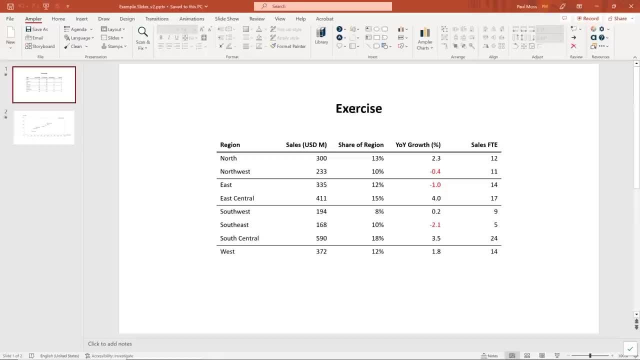 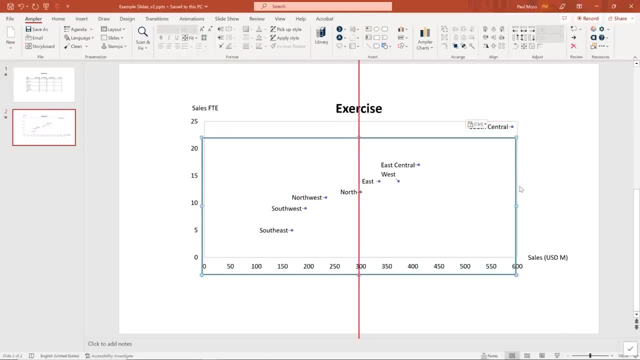 message. So the first thing we're going to do is just add a simple title here. That's going to give us bang for the buck in terms of effort. Let's move this chart down a little bit, All right? so let's just put a simple title in here: More sales. FTE tend to need to hire sales. 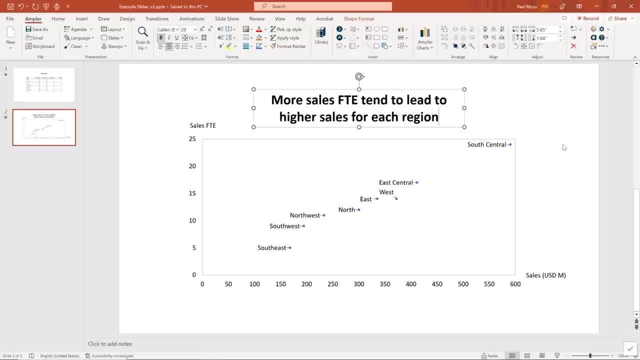 for each region. Probably a better title out there, but we'll just stick with this one. It's pretty simple, But really the main focus of this is to emphasize the message in the chart. Now the thing we're going to do is just add a simple title here. So let's just add a simple title here. 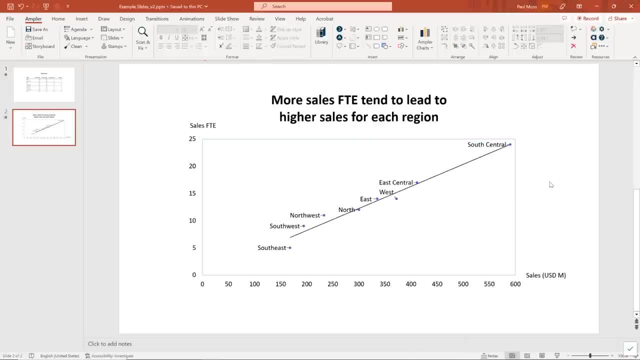 And we're going to put a simple title here, And we're going to put a simple title here And we're going to do here is: we can add a trend line. this is going to help emphasize that this is a positively correlated relationship between these two variables. all right, 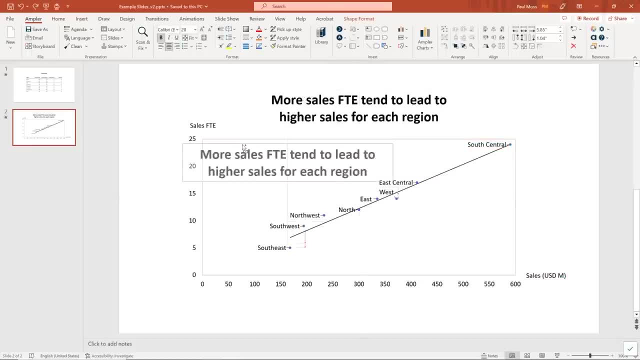 just to make sure we're being comprehensive, let's include a little subtitle here. let's say: sales FTE versus total sales USD the year here, just to be comprehensive, a little smaller italicize. there we go. so now we have the basics of our chart in place. it's really just about removing clutter and the good. 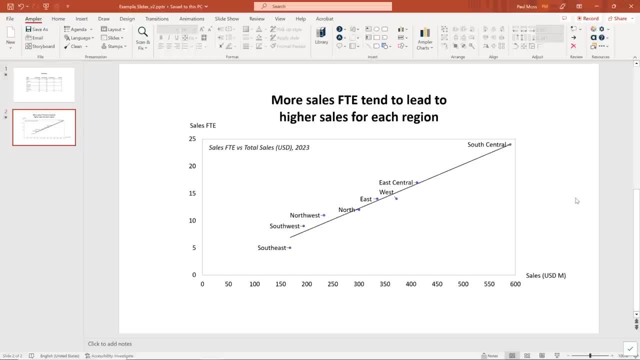 thing is with a chart like this, it's kind of already decluttered, so we can't really remove the axes here. I think that would take away from the effectiveness of this chart, it being a scatterplot. we could probably remove the labels, but they don't clutter the chart too much, so I